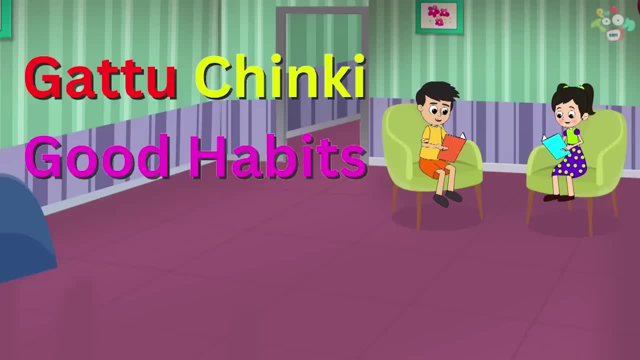 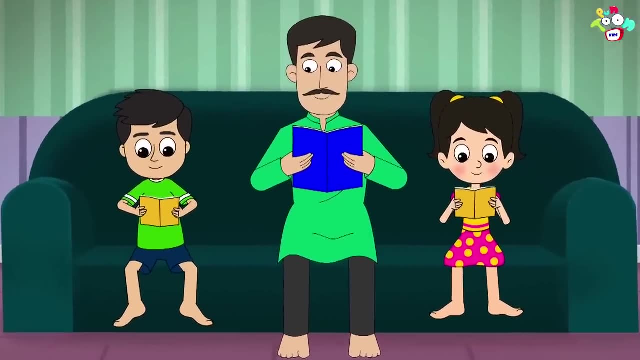 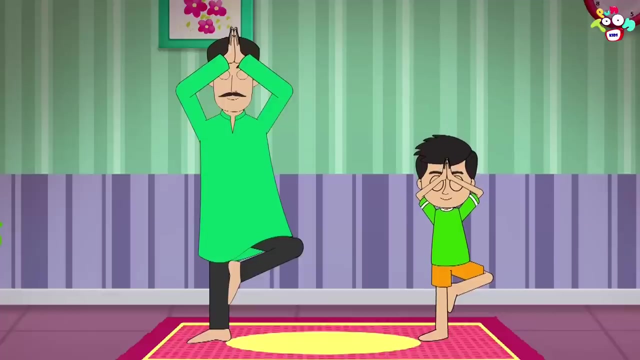 Gattu Chinki's Good Habits. We all know that children learn good and bad habits by watching, But sometimes it becomes necessary for children to learn to differentiate between good and bad habits. Today, a guest lecture has been organized in the school. 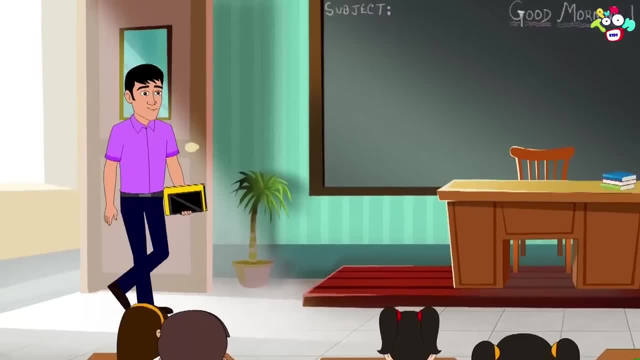 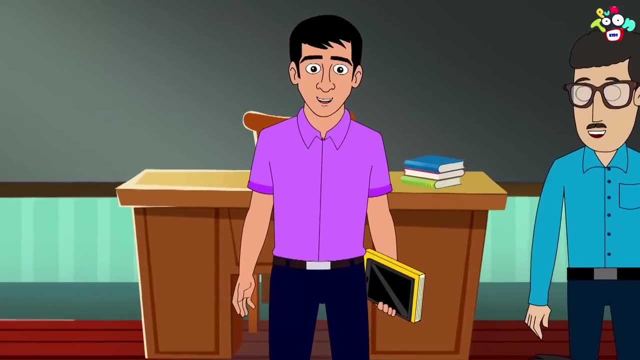 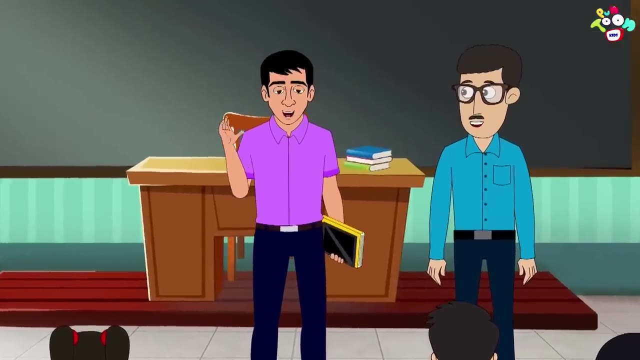 All the children are waiting for him. and then he entered the class. The motivator was very young and he had some books and a big tab in his hand And the children got very excited seeing him. Good morning everyone. Today I will discuss with everyone about good habits and bad habits. 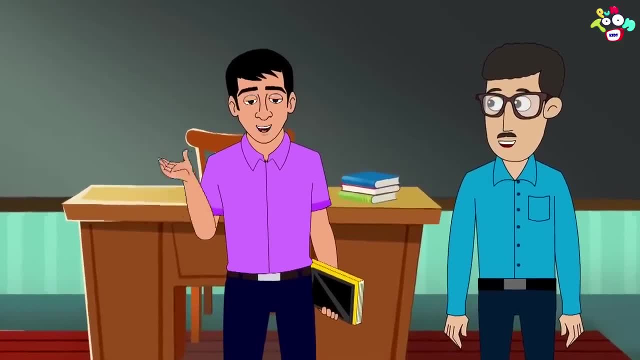 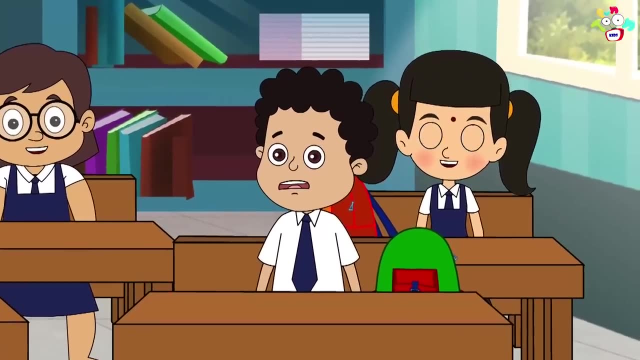 First of all, you all will tell me about your good habits. Let's start with you. Sir extended his hand towards Bunty And suddenly Bunty was asked to speak And Bunty started hesitantly. But My good good habit is: 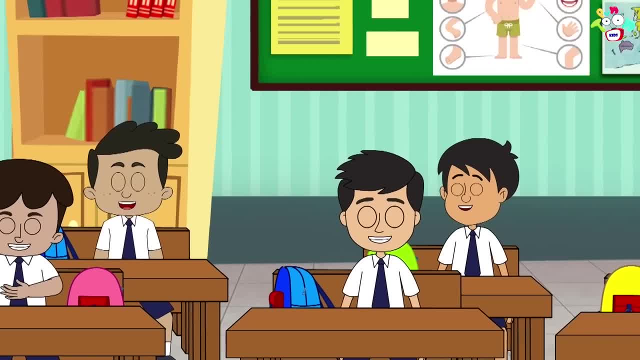 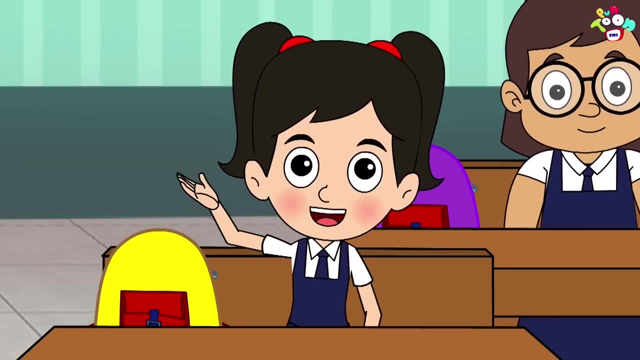 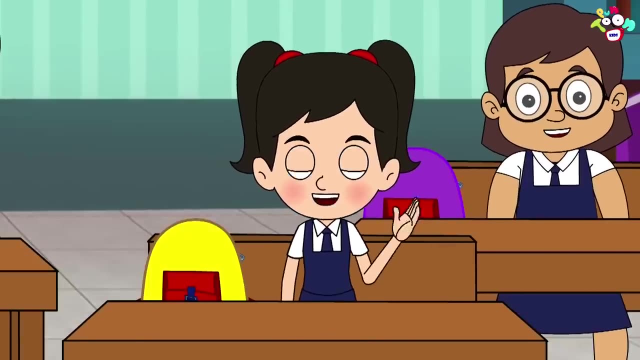 I, I like to eat chocolates. The class laughed at Bunty's answer. Okay, next, Mom and dad says that completing school homework is my good habit. Sir, let me share one more good habit of Gattu. Yes, of course. 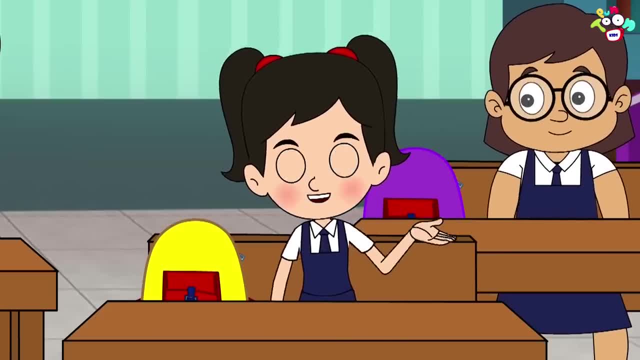 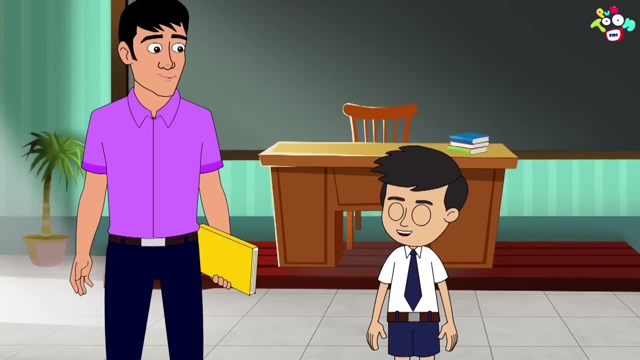 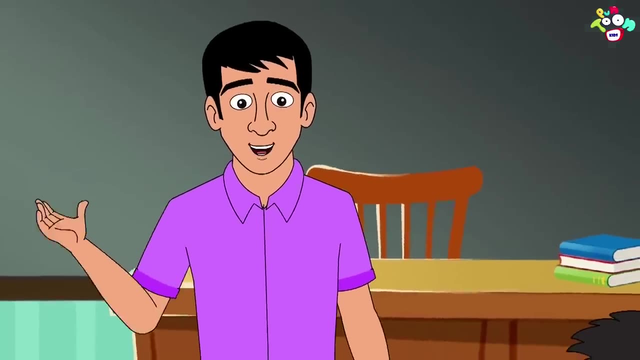 Sir Gattu's good habit is that he always helps me doing my homework And many times Gattu completes my entire homework. Yes, yes, sir, So many times I have completed Chinky's homework. Look, kids, all of you told me your good habits. 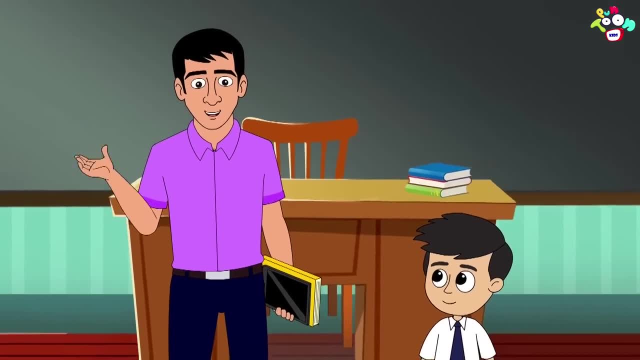 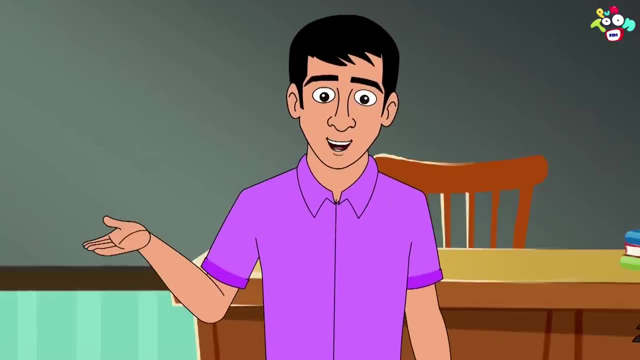 But see here: Gattu completes Chinky's homework along with his own, Which Gattu is calling a good habit. It will be a good habit for Gattu, But it is not a good habit for Chinky at all. 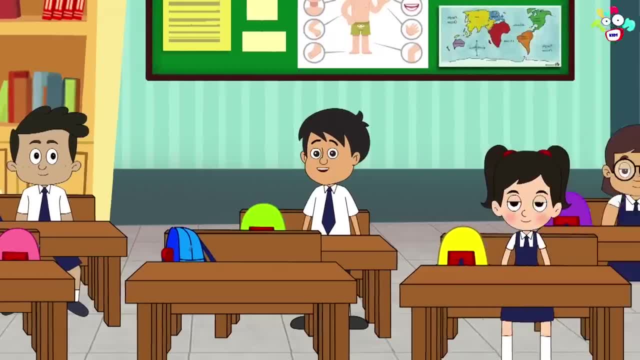 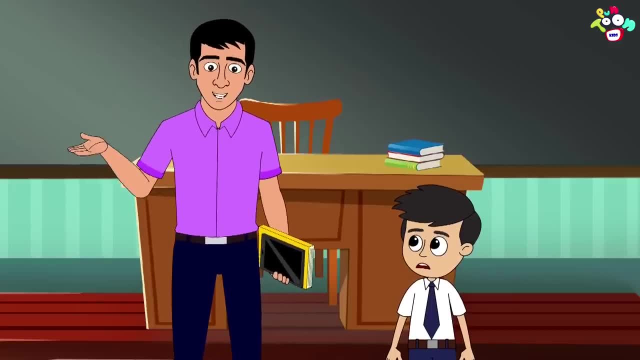 Rather it would be called a bad habit. Everyone started listening to sir carefully. We should all do our works by ourselves. Come on, kids, let me tell you my story. As a child, both my brother and I had a habit of eating chocolates. 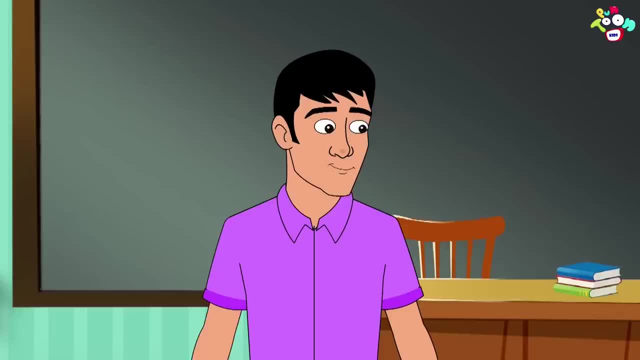 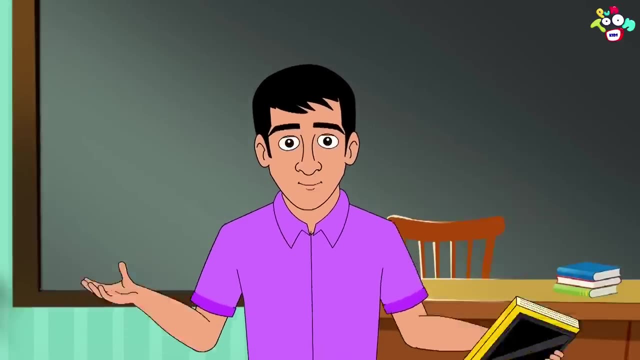 But, sir, eating chocolates is a good habit, isn't it? Yes, son, But we would ask for chocolates from the guests. Then our father told us, If we want chocolates, then we should go to the garden and water the plants first. 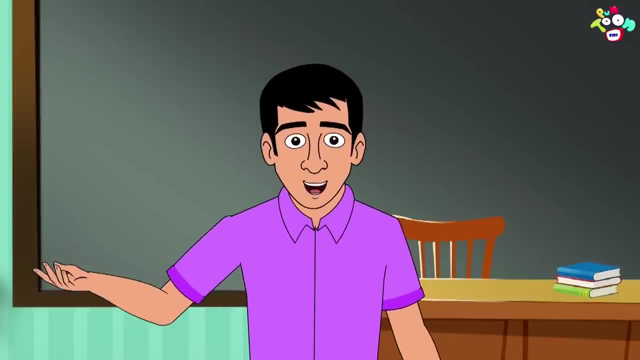 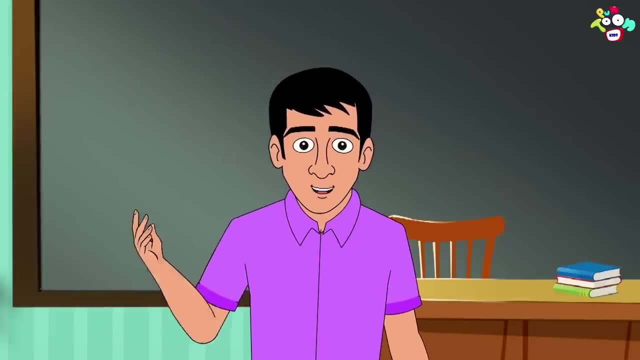 Only then we will get chocolates, And at that time our house was on the 7th floor. We would come down from the 7th floor for chocolates, water the plants and then only get chocolates. The children were listening carefully to, sir. 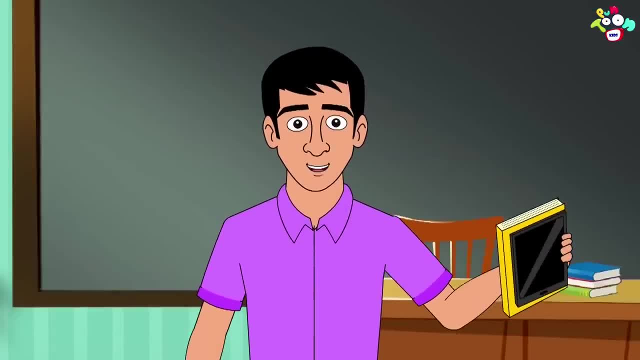 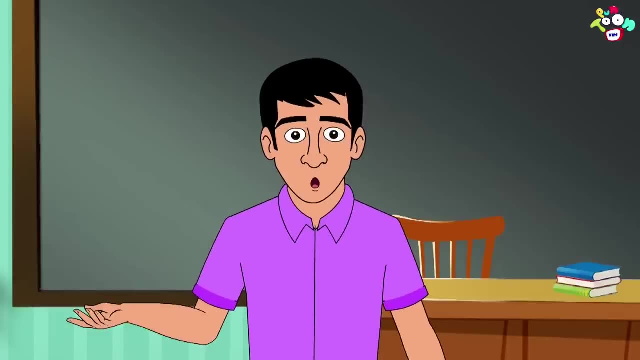 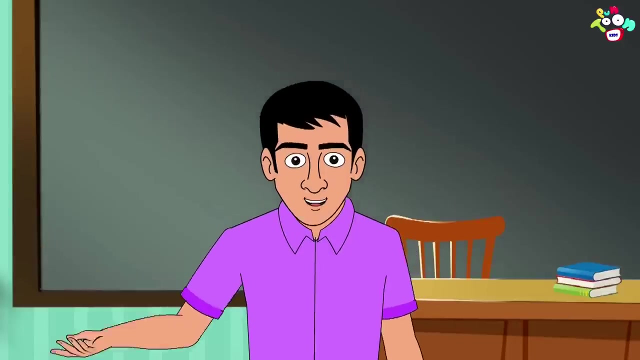 In this way. when we got chocolate every day, we got bored of eating chocolates And later we stopped eating chocolates. But we got into the habit of watering plants And we have been watering our garden till this date. Yes, sir, This is how we got into a good habit. 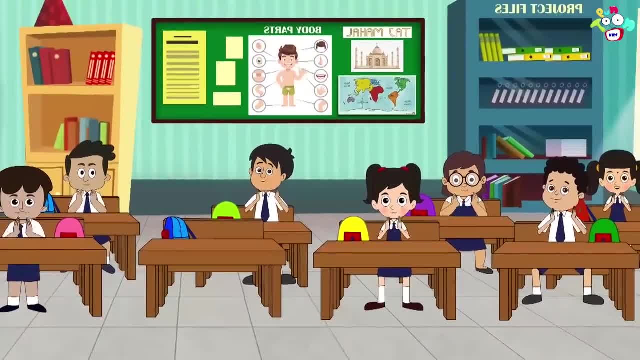 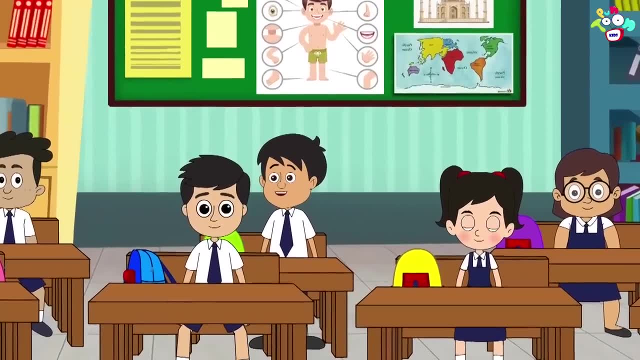 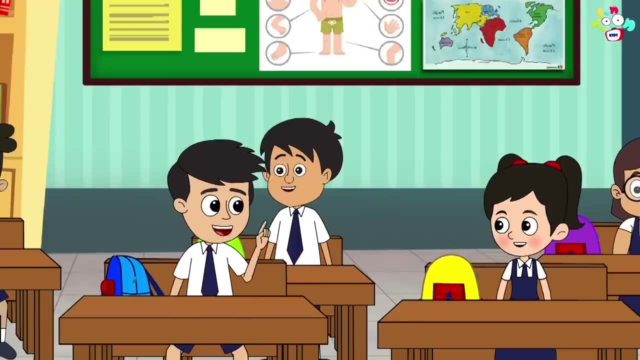 All the children were listening to the sir so attentively that all the children clapped for him. After the guest lecture was over, all the children started discussing with each other about good and bad habits. Grandma always says that if we have good habit, we become successful in life. 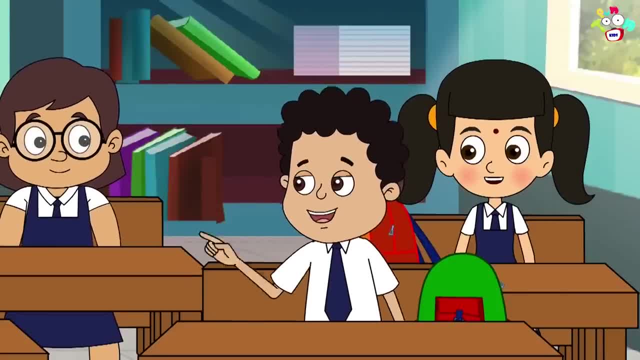 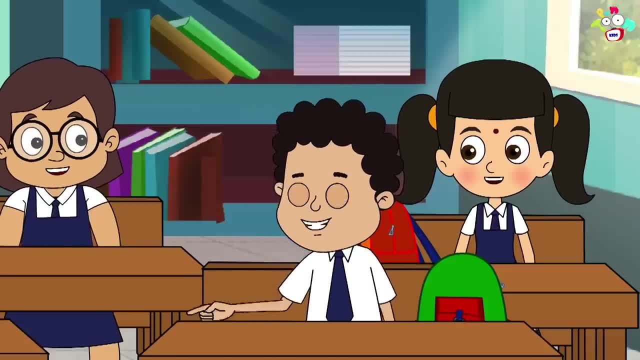 Now, just like sir, I will also water the plants every day. Only then I will eat chocolate. In this way I will also get into a good habit, But I will not give up eating chocolates. Everyone laughed at Bunty's statement. 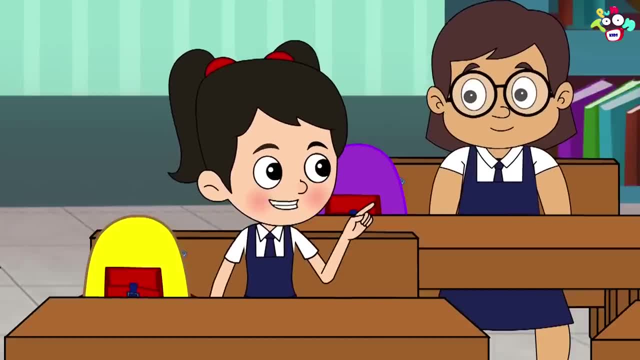 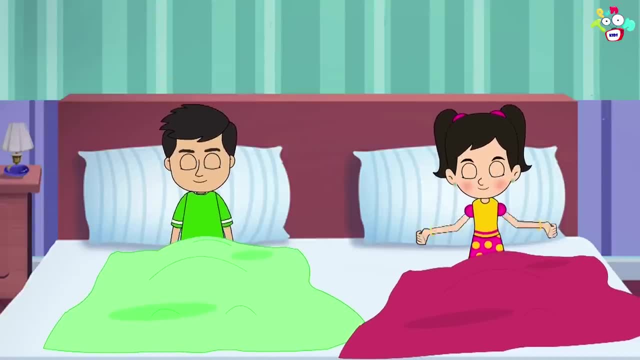 Yes, we should always be like a good child. We should not bother our parents too much. Well said, Chinki. The next morning, Gattu and Chinki got up early and sat on the bed before mom got up And started worshipping the earth. 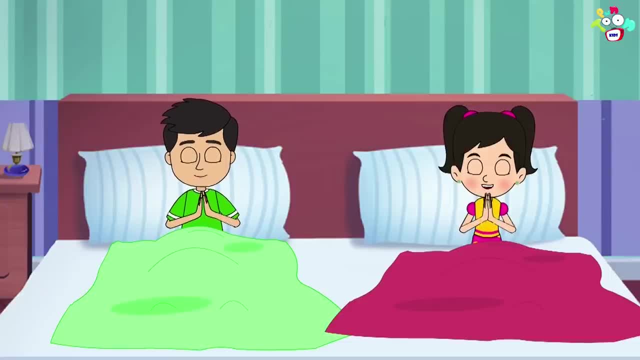 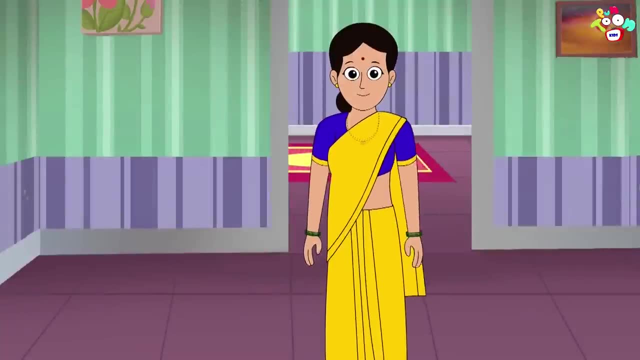 Karakre vaste Lakshmiya Karvatye, Saraswati, Anmoletu Govinda, Prabhate Kar Darshanam. Mom came out of the kitchen after hearing the voices of Gattu and Chinki. Oh wow, Gattu and Chinki. 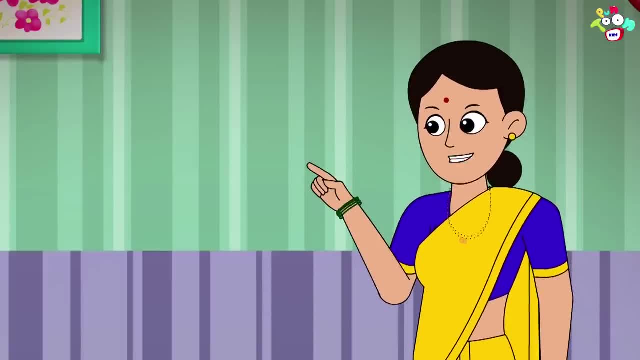 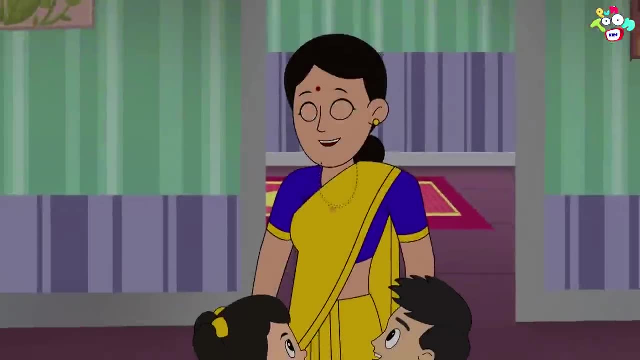 You got up early and you both prayed together. What's the matter? Gattu and Chinki got down from the bed and went straight to their mom and hugged. Mom got happy on this gesture of Gattu and Chinki. Gattu and Chinki took a bath and got ready. 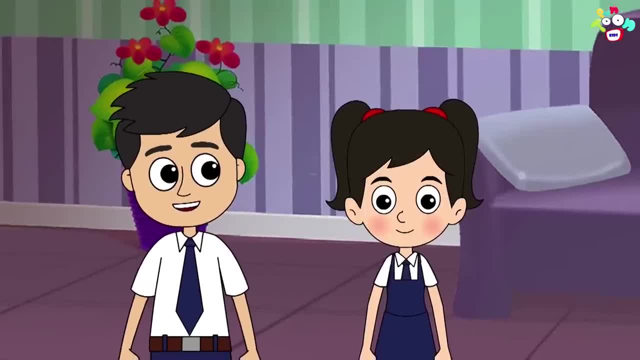 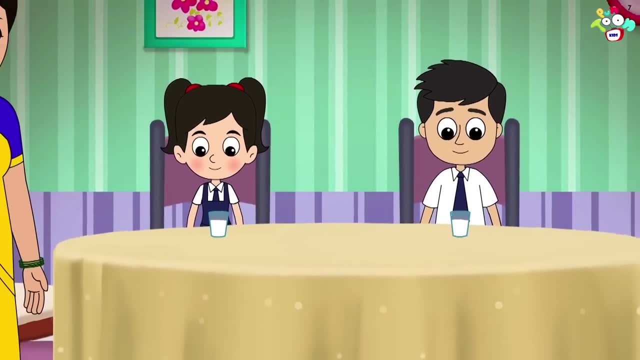 Today mom did not have to chase after Gattu and Chinki Without saying anything. Gattu and Chinki got ready quickly. Gattu and Chinki were sitting at the breakfast table. Mom hands over a glass of milk to both Gattu and Chinki. 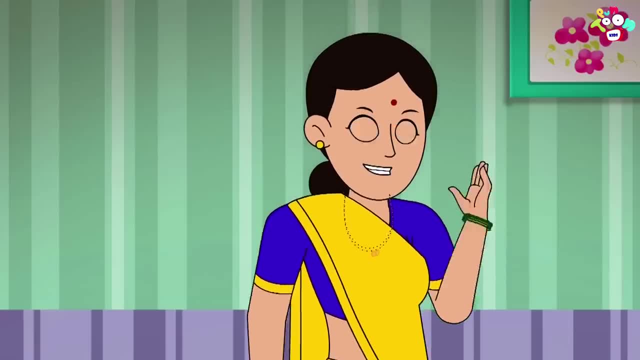 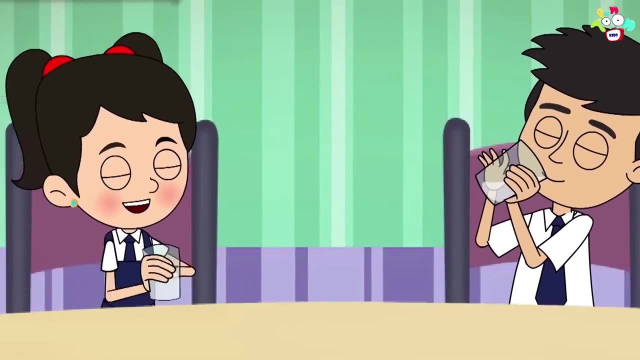 Gattu and Chinki, don't pretend to drink milk like everyday. You both have to finish the milk like good kids. Yes, mom, let me finish now. Gattu and Chinki both finished their glasses of milk in no time. 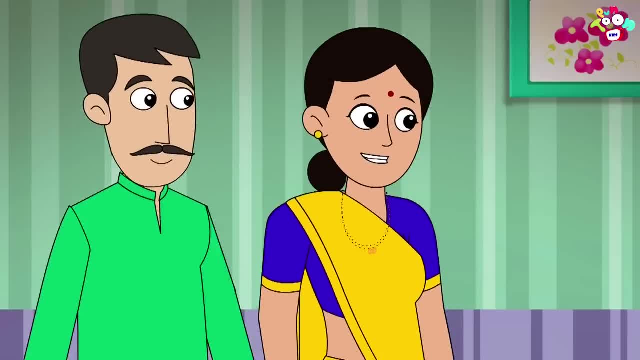 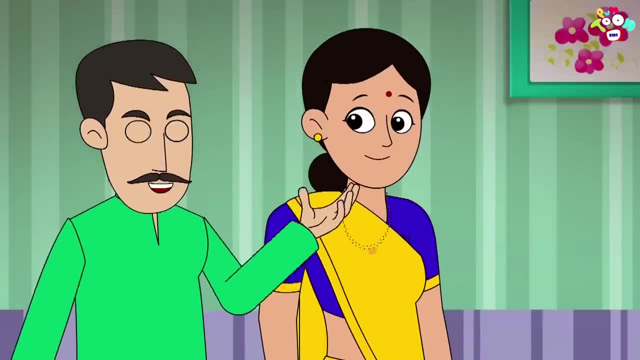 Mom and dad were surprised to see this. What's the matter? Gattu and Chinki, Both of you are behaving like good children. I am very happy to see you both behave like this today. Thank you, dad. It is a good habit to listen to elders. 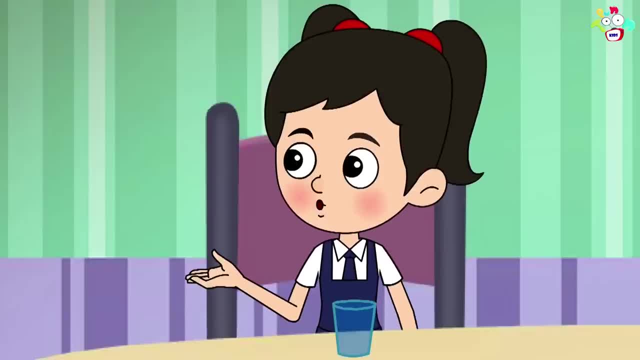 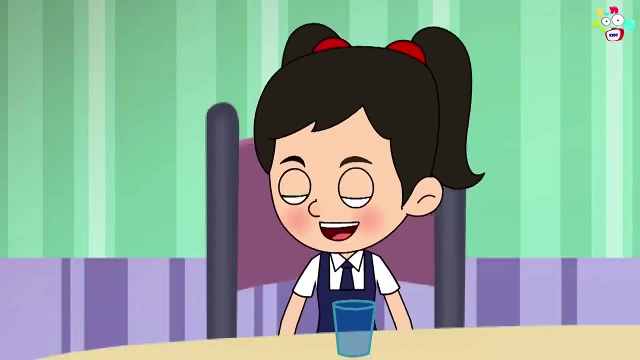 Now we will finish our milk like this everyday And we will not bother you. Very good, Gattu and Chinki, But, son, everyday you leave after 10 minutes. Yes, mom, but we have to reach school before time. This is a good habit. 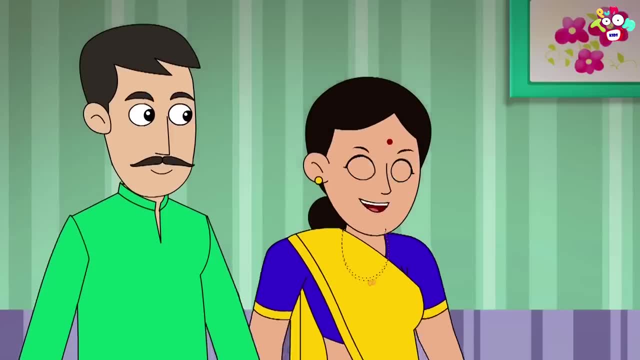 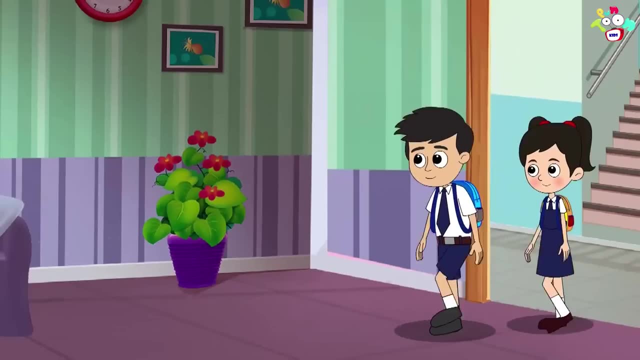 Because of which we will not be late in school. See how intelligent my children are. Gattu and Chinki left for school with dad. Gattu and Chinki returned home in the evening. Both of them put their school bags, their shoes, in the right place. 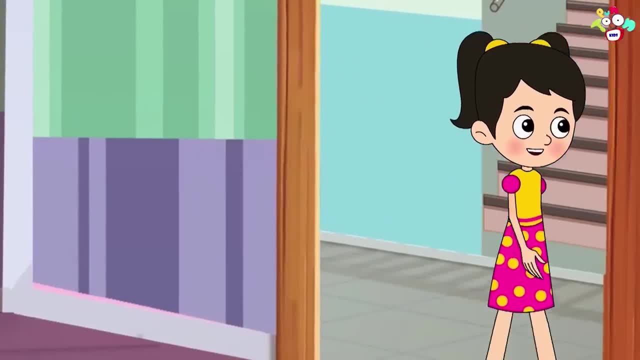 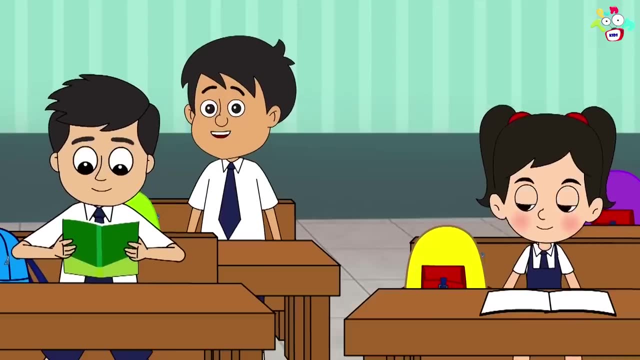 And after changing their uniforms, both of them went downstairs to play. Similarly, Gattu and Chinki used to get up early everyday, finish their milk And then, after studying well in school, they would go to play after returning in the evening. 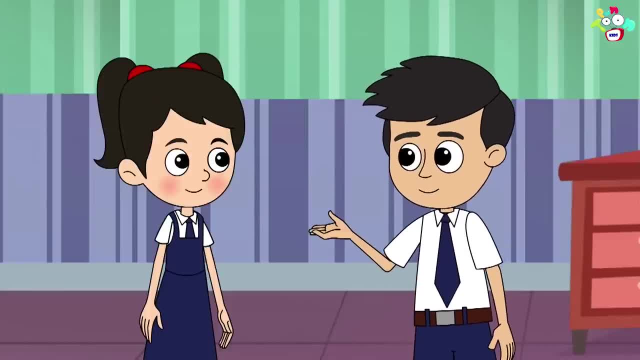 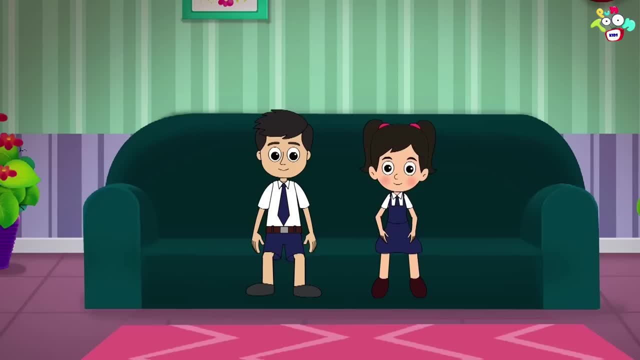 Chinki, there is time before we leave for school, So let's watch TV. Yes, Gattu, there is time And a new cartoon show has also come on the TV. Let's watch. Gattu and Chinki sat in front of the TV and left for school with father when it was time to go to the school. 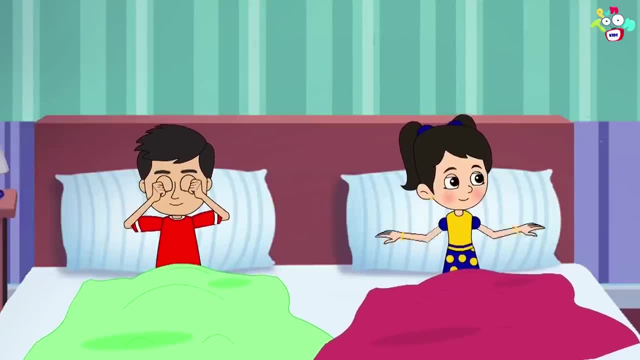 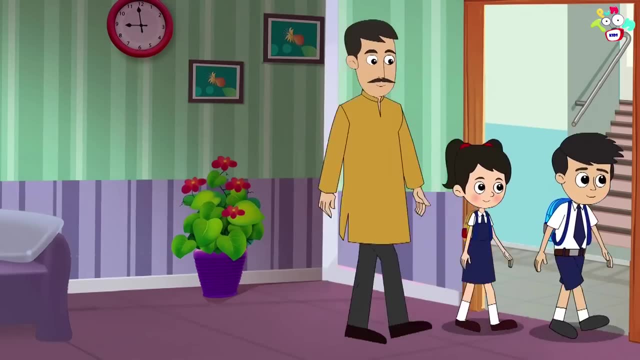 Mom noticed Gattu and Chinki Everyday. Gattu and Chinki would get up early, sit in front of the TV as soon as they get up, When it was time for school, they would leave for school. Today again, Gattu and Chinki sat in front of the TV. 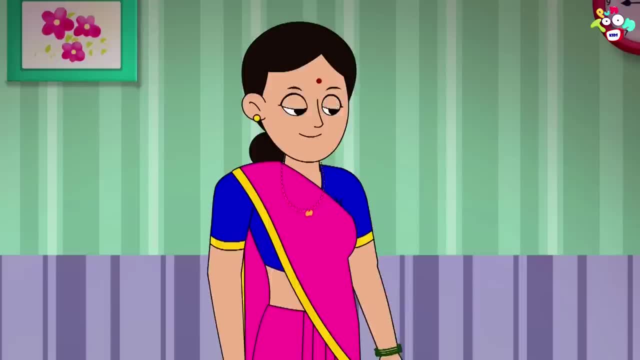 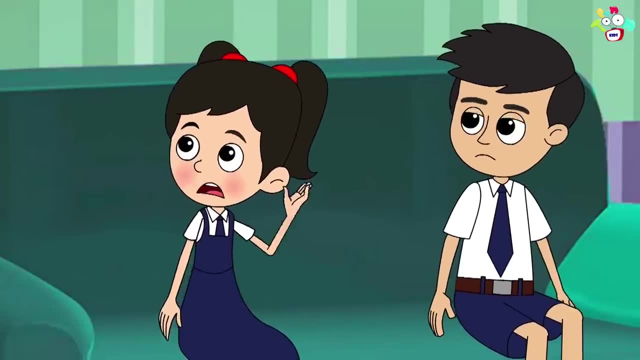 Gattu and Chinki sat in front of the TV before school. Gattu and Chinki, why are you children spoiling your habit by sitting in front of the TV early in the morning? What mom? you too. We get up so early and then there is time to go to school.